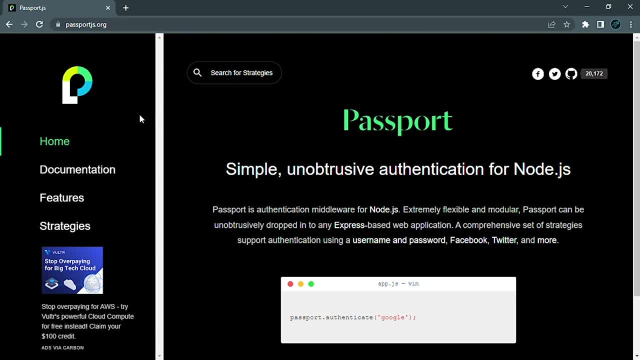 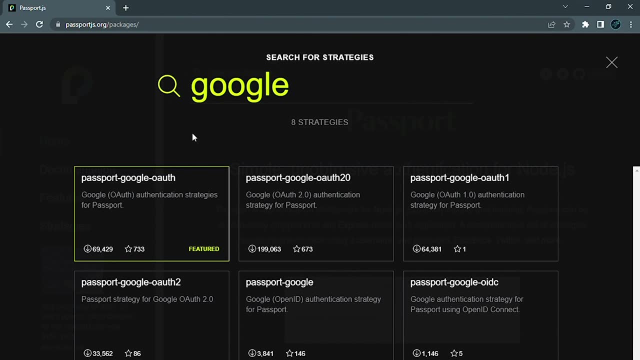 To integrate google authentication in our application. we gonna use passport module, which is a middleware for nodejs that makes easy to implement authentication and authorization For google authentication. we need a strategy: click on strategy link and search for google. we gonna use passport google earth 2.0 because lots of people has downloaded it. 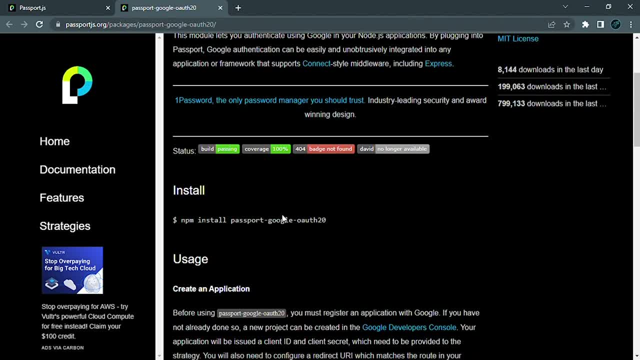 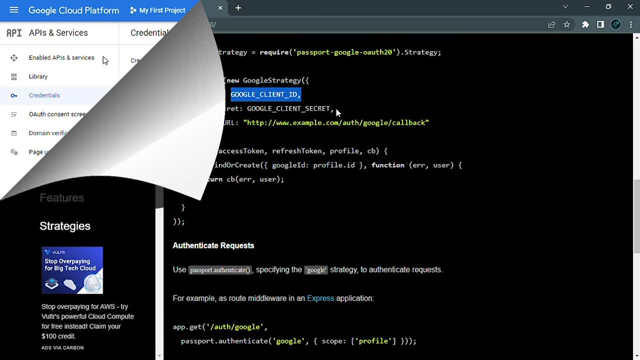 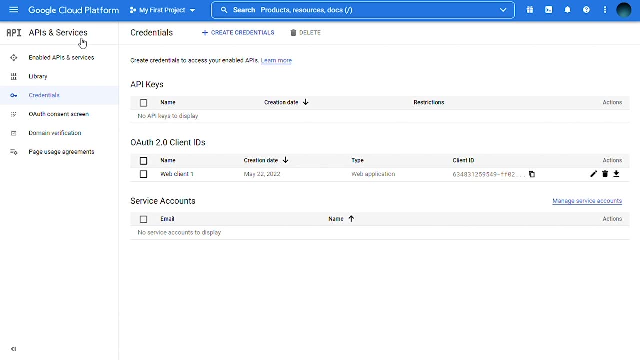 If you have encountered any error, please refer to this doc, which is very good actually, but to use google strategy we need to have google client id and secret key. Go to google cloud website and create your account and then, in apis and services tab, first create earth consent screen and then, in credentials tabs, click on create credentials. 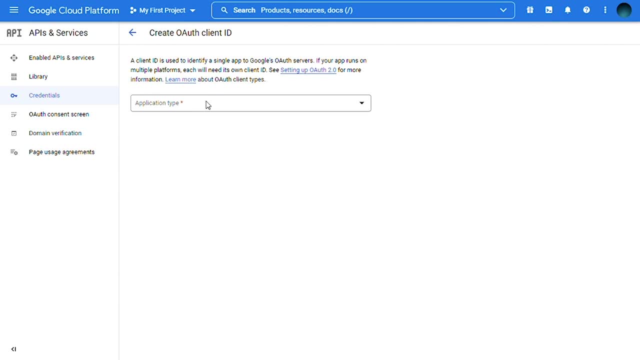 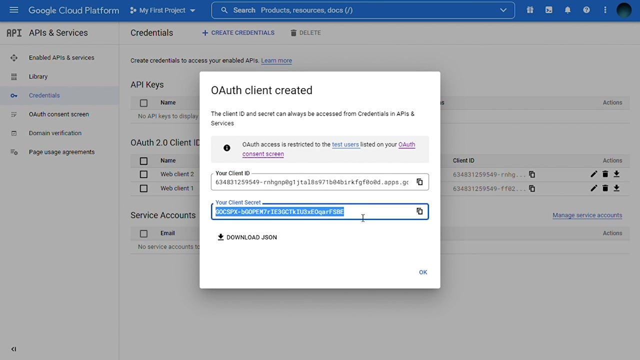 and select earth client id. Application type will be web application. Add authorized redirect url. add url http//localhost3000 and add one more url: localhost88. earth google callback. Then click on save button. Now copy your client id, secret id and save it somewhere, or download json file. 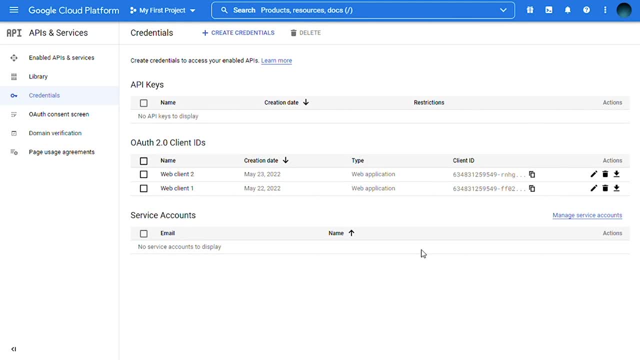 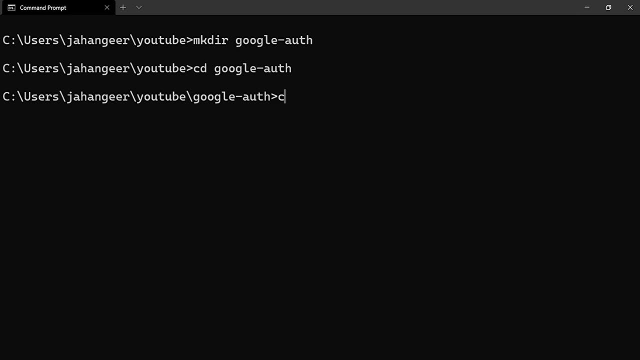 Now we have our client id and secret id. Let's open up a command prompt. First, let's create a folder named google earth and then navigate into it. In this folder, create a folder named server and then navigate into it. Here we gonna initialize this project with npm, with default values. 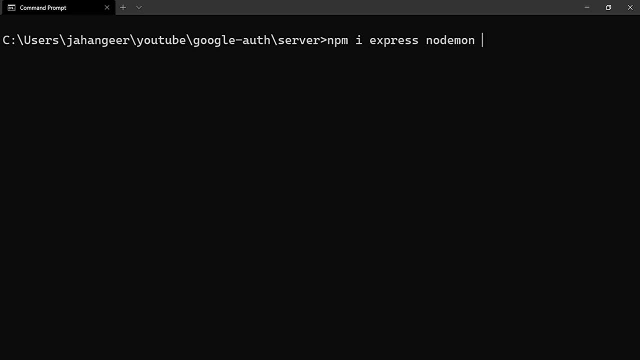 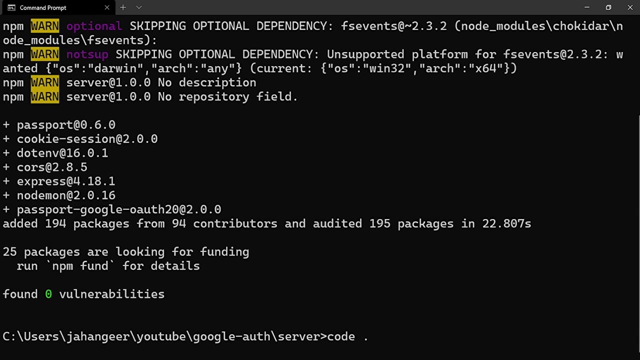 After initializing, let's install dependencies we need in this project, which are express: nodemon course, dotenv passport, passport google earth 2.0 and password google earth 2.0 cookie session. After installing dependencies, open this project in VS code. 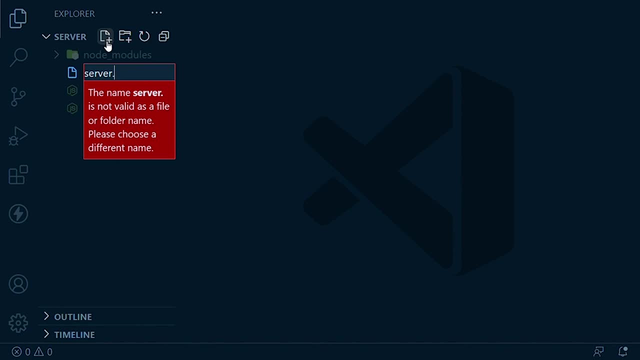 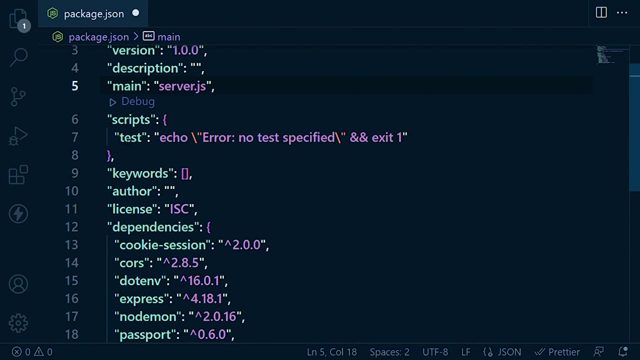 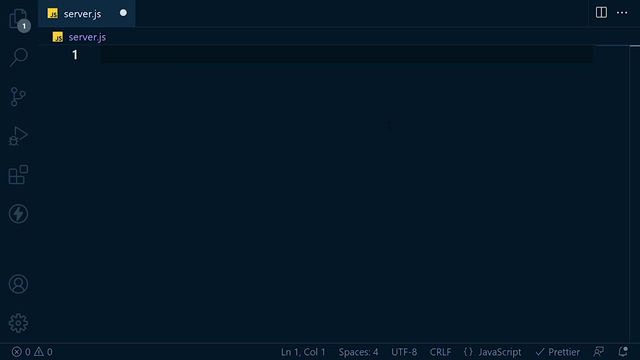 In root directory create a file named serverjs. then in packagejson change main file to be serverjs. In scripts- test scripts- and add start script nodemon serverjs. save this file and open serverjs file. in this file let's import dot env module which we gonna use for accessing environment variables. 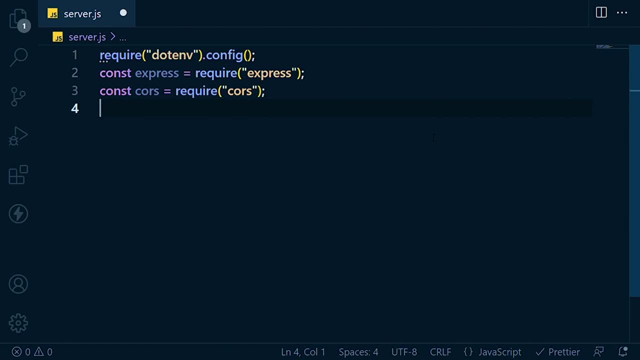 then import express module, course module, passport module and cookie session module. call express function and save its instance in app variable. we're gonna use cookie sessions here. i'm gonna name it session keys will be cyber wool and max age will be this much, then, we will using. 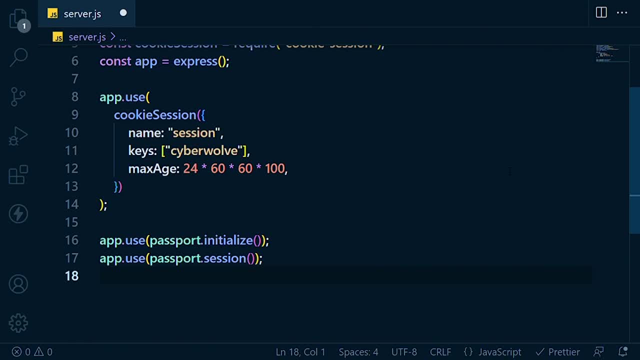 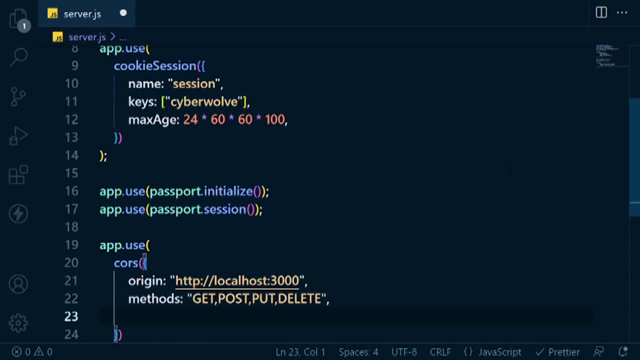 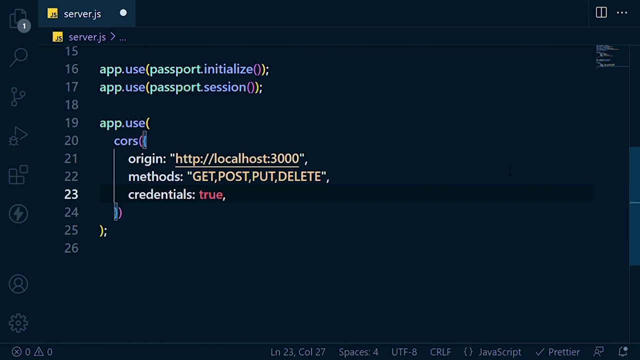 passport and initialize it and we also used passport session after that. we use quotes. origin will be our front-end ul. methods which we gonna allow are: get, post put and delete and credentials are required. so set it to be true. define port variable which can be environmental port. 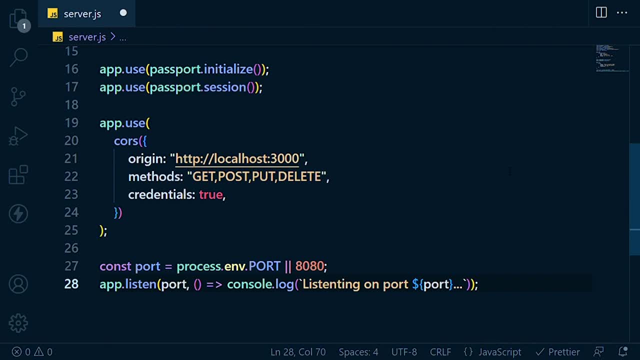 or you can put the port as the default. how to initialize port and cord is given in this article. what were the missionals of Nord chops? five components are required to will show the Я собирать. and Then we listen. our app on port and console log listening on port. 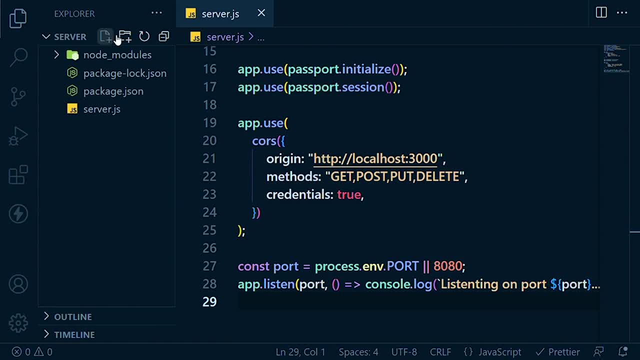 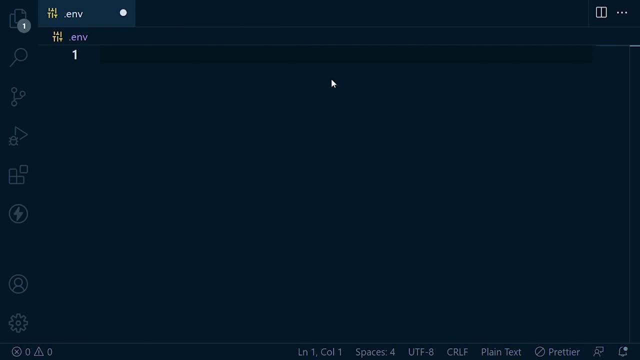 Save this file and, in root directory, create env file. In this file, add your google client id, google secret id and client url, which in my case, I am running it on port 3000.. After adding details, save this file and create passportjs file in root directory. 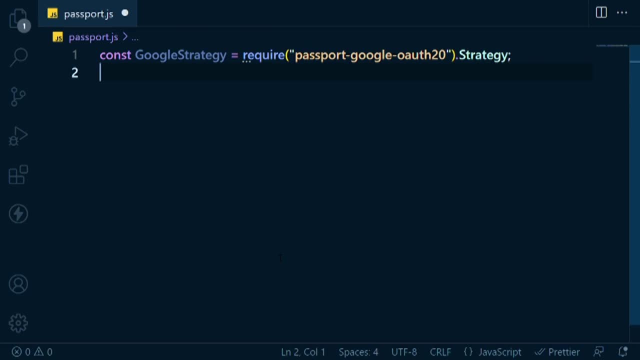 In this file. import strategy from passport google earth 2.0 module and save its instance in a google strategy variable. Then import passport module In passportuse. add new google strategy. Inside that object add your client id, client secret, callback url and scope. 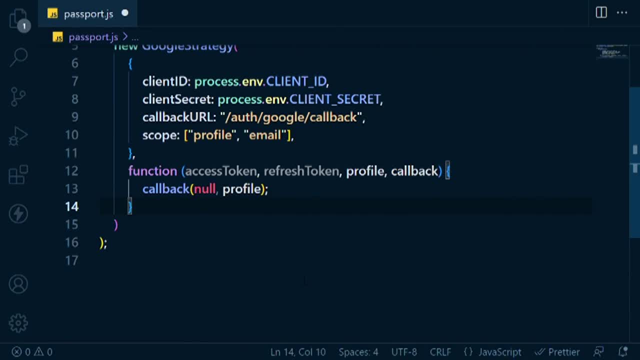 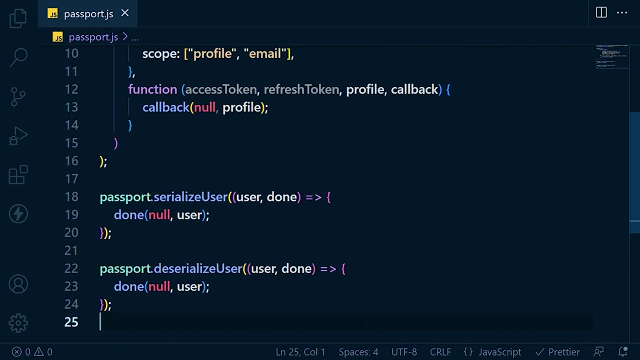 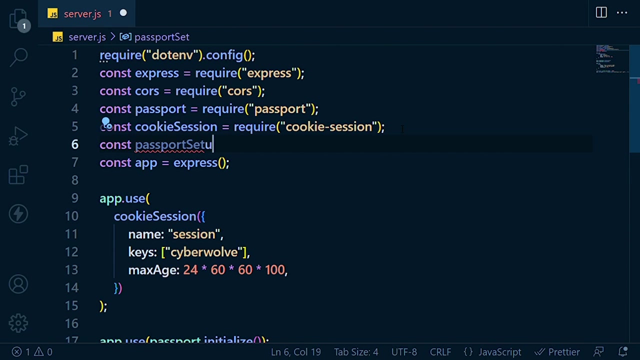 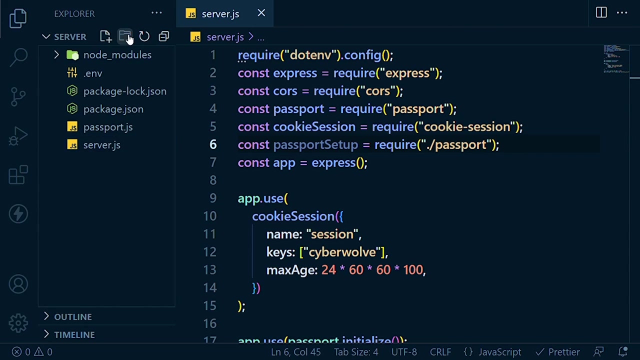 For callback response. I am just gonna return profile details. we are using cookie sessions, so we need to serialize user and deserialize user. Let's save this file now and import it in serverjs file. After importing, create routes folder in root directory. Inside that folder, create earthjs file. 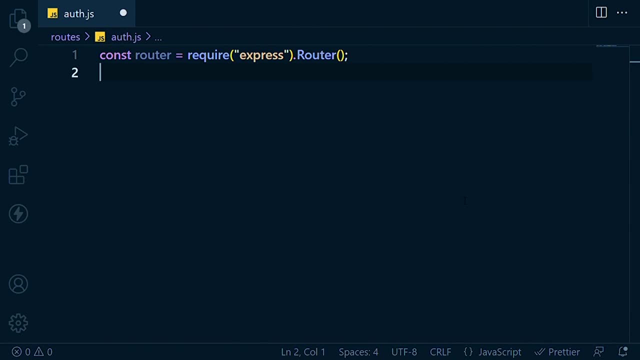 In this file: import router from express module and import passport module. here also Let's add get api with endpoint google slash callback And add passportauthenticate and add google init. If it's success, we redirect to home url. If it's failure, we redirect to login- failed route. 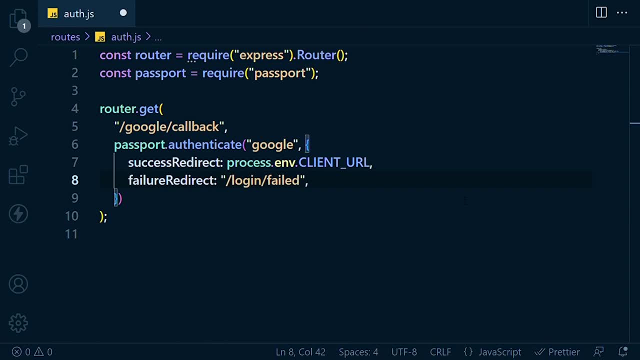 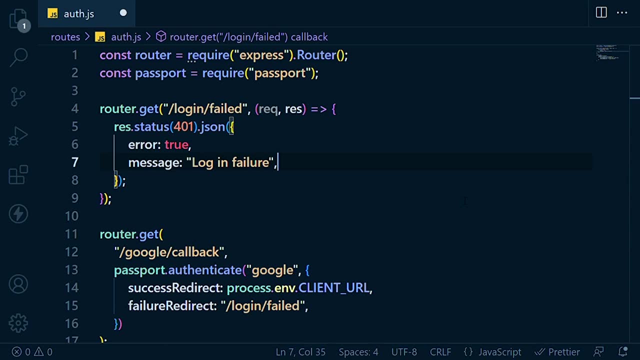 We haven't created that route yet. Let's create now. It's gonna be a get api with endpoint login slash failed. We just gonna return With status code of 401.. And json object Error. to be true, Message will be login failure. 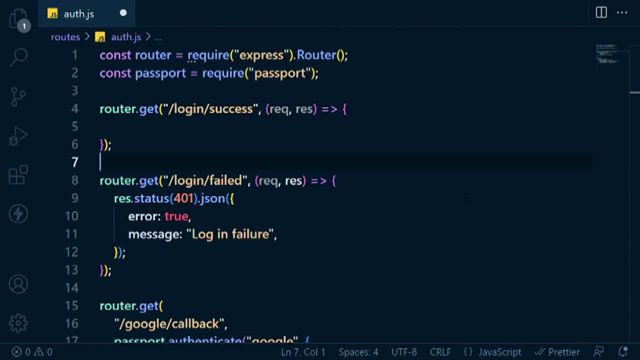 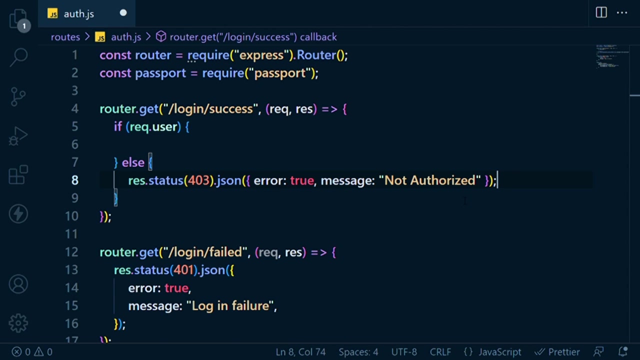 Let's add a get api with endpoint login slash success, which we call it- from frontend, to check whether the user logged in or not. Passport will verify user by comparing session from frontend and backend. If requestuser does not exist, we return with response with status code of 403.. 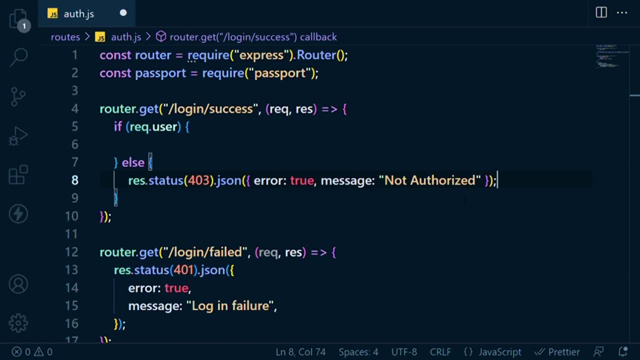 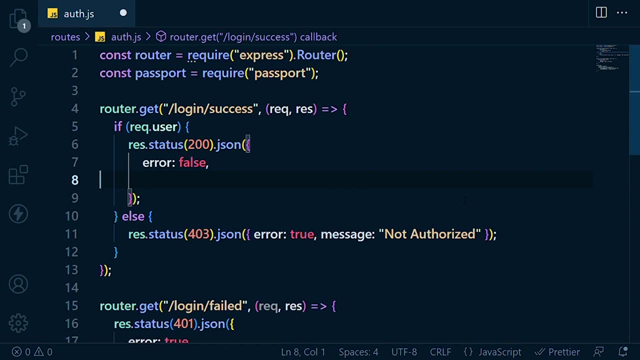 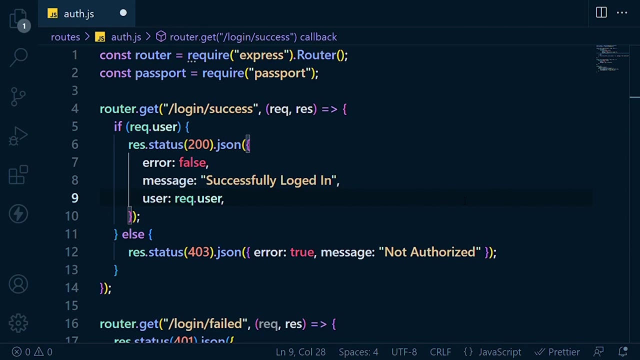 And json object will be error to be true Message will be not authorized. If user exists, we return response with status code of 200. And json object will be error will be false Message. successfully logged in User to be requestuser. We gonna add another get api with endpoint slash google. 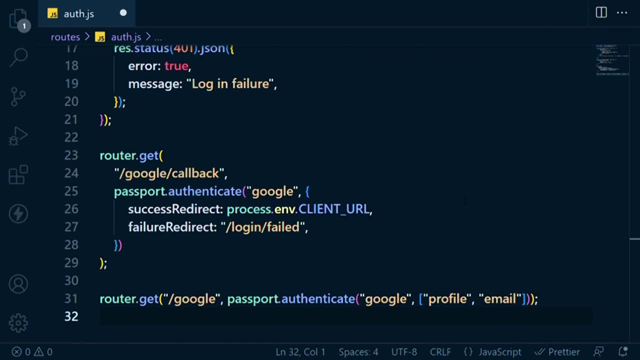 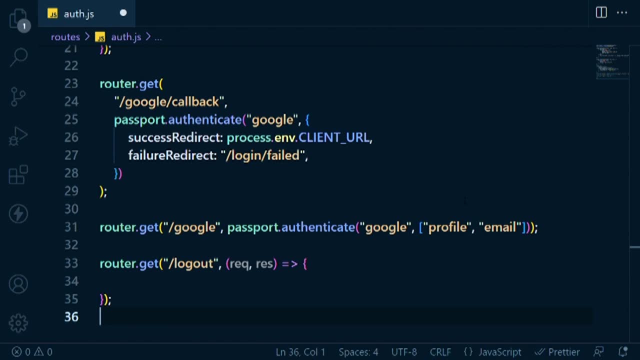 And add passportauthenticate method Inside that provide google and scope. Let's add last api with endpoint slash logout In that function, Call requestlogout method and then redirect to client url. After adding all these apis, let's export this router and save this file. 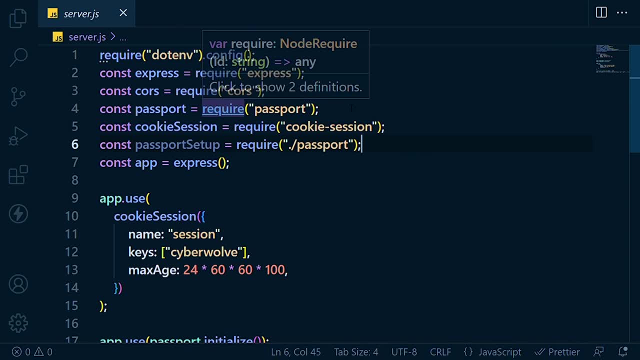 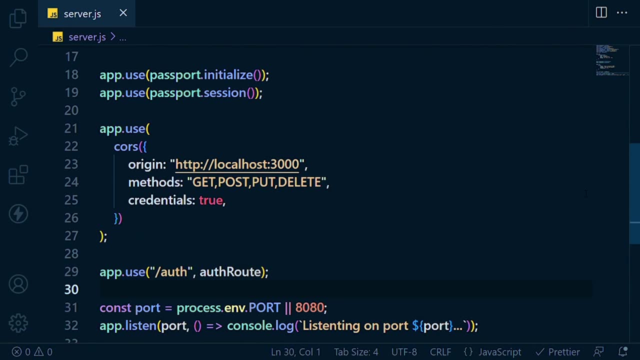 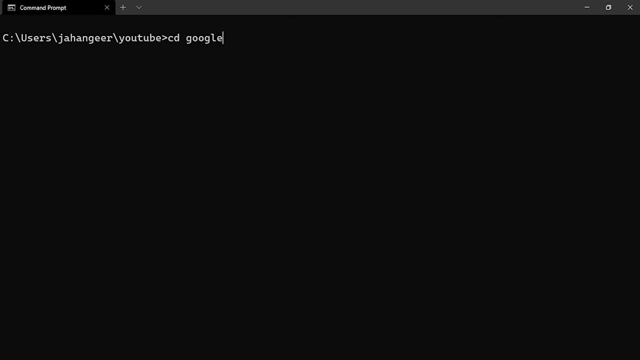 In serverjs. import auth routes and use them at endpoint: slash auth. After configuring routes, let's save this file. Ok, guys, our backend part is completed. Now let's focus on frontend. Open up a command prompt inside our project folder: Run command npx- run. 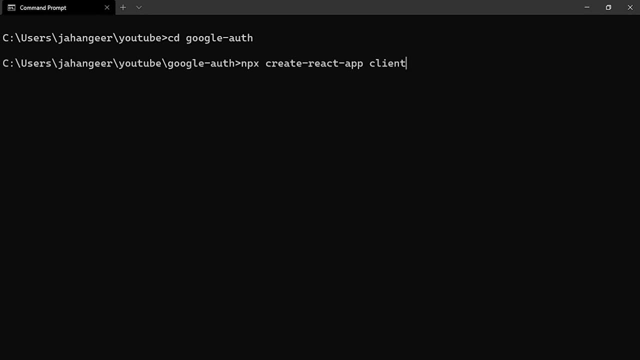 Run command: npx- create reactapp. I am naming it client. You can name it anything you want. It's gonna take a while to create, So I will fast forward video. After creating react application successfully, Let's navigate into it. Here we gonna download some dependencies we need in this project, which are xios and react. 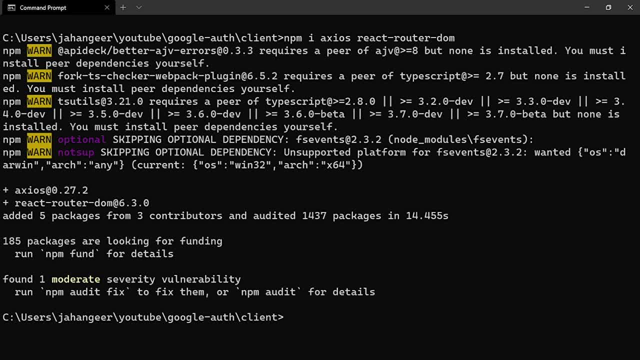 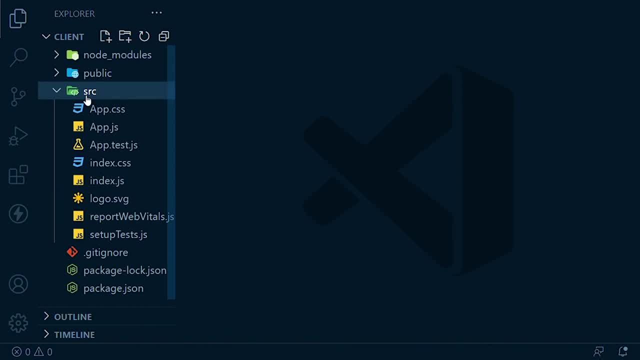 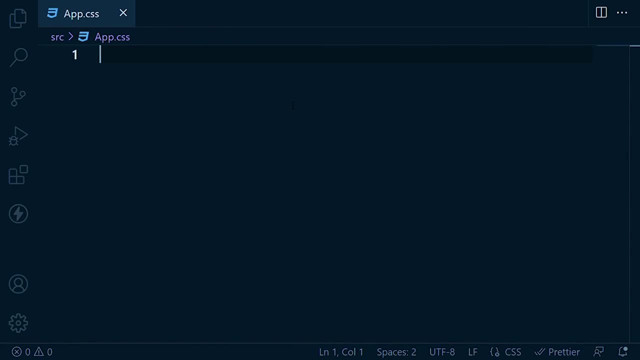 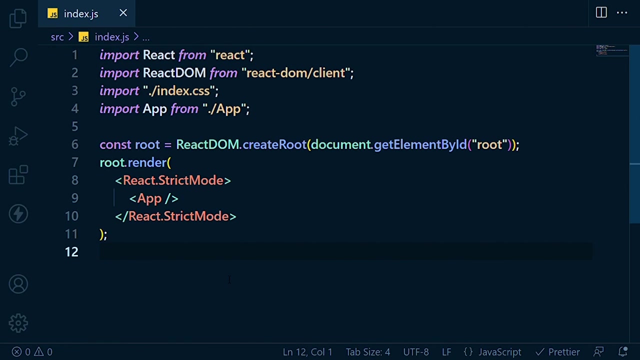 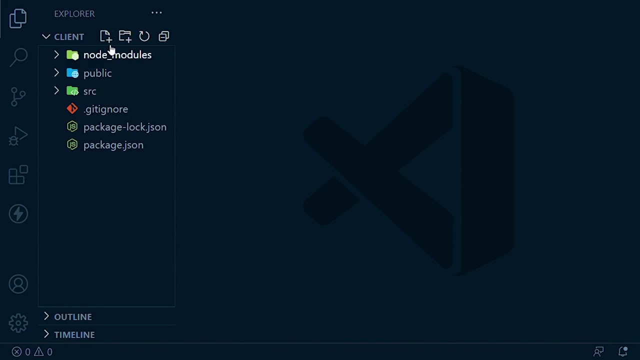 router DOM. After installing dependencies, open this project in vs code. Before we jump into writing, Let's remove unwanted files and code first. Now our project looks clean, Let's create env file in root directory. In this file let's add our backend url, which, in my case, I am running it on port 8080.. 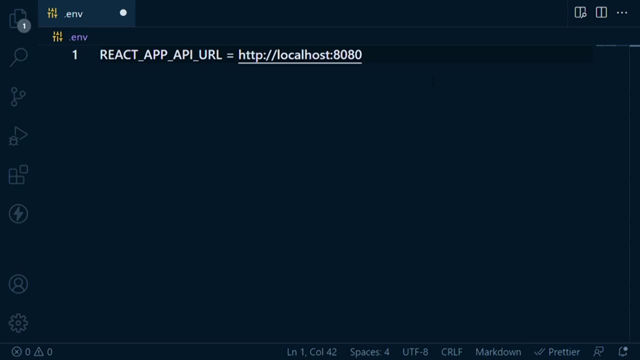 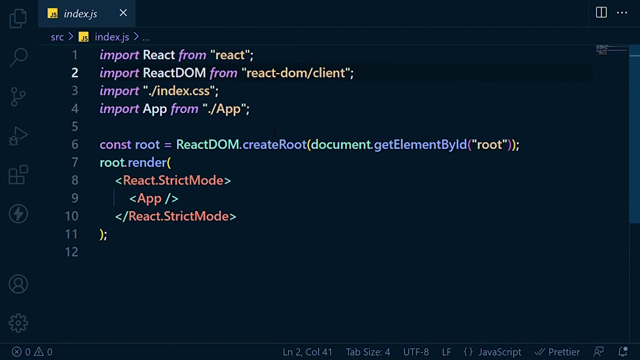 Make sure to append reactapp for every environment variable you use. If you won't append, then you can't access environment variables. After adding api url, Save this file And open indexjs file In this file. import browser router from react router DOM. 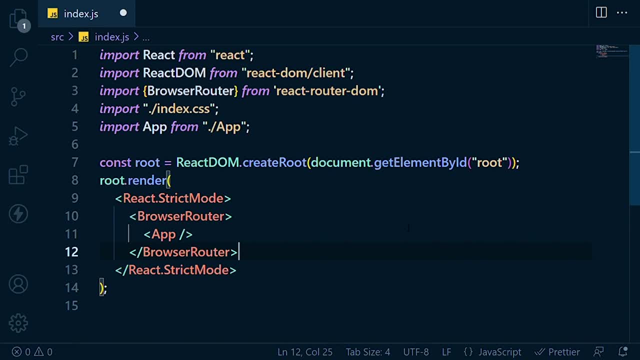 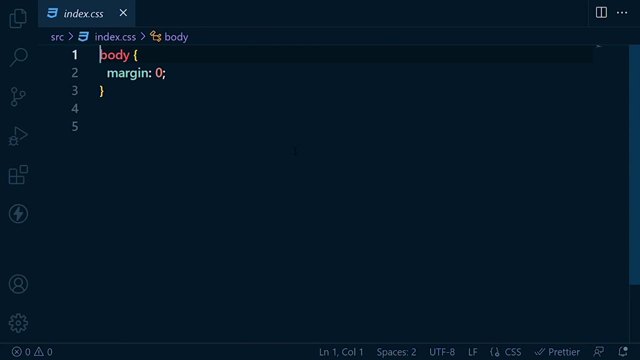 Then wrap it around app component. After making changes, save this file and open indexcss file. In this file, import popin's font style from google fonts. Check out google fonts website. you will find this url Or copy it from github repo. Add font family to be popins and sans serif. 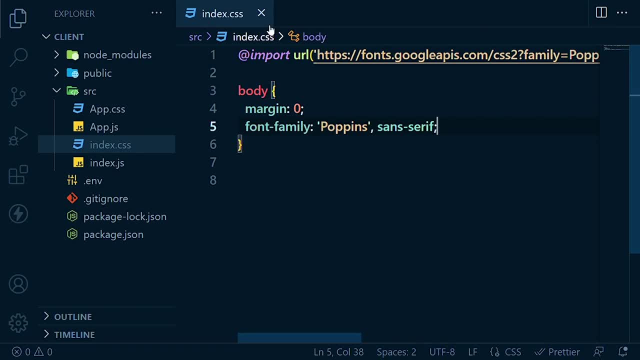 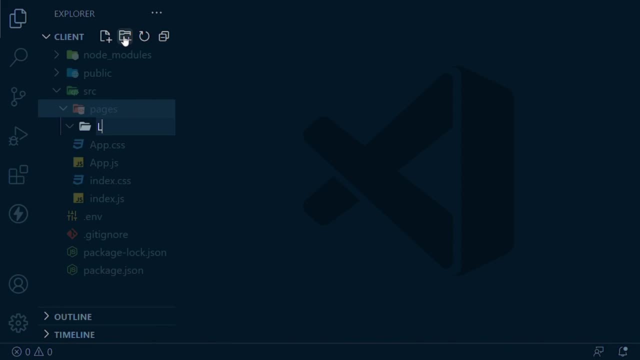 Save this file now. Then in source directory create folder named pages Inside that folder. create login folder Inside that folder. create indexjsx file and stylesmodulecss file In this file import link from react router DOM, Then import styles from stylesmodulecss. 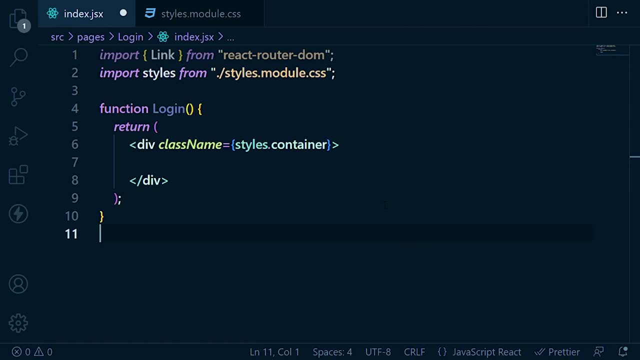 Create a function which returns div element and name it login, And don't forget to export it. Inside the div, add a heading login form And add div with class name form container. Inside the div, add two more divs with class names, left and right. 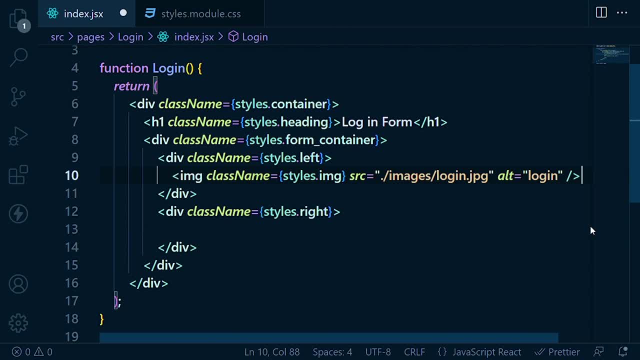 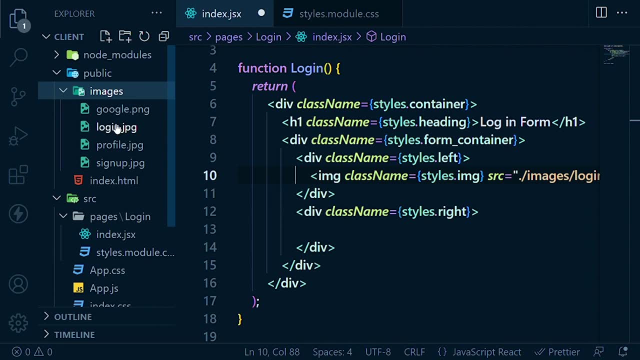 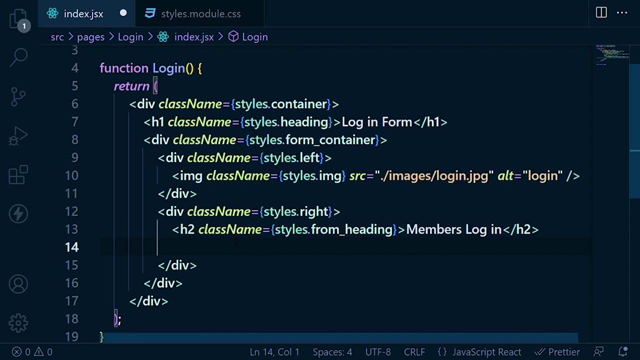 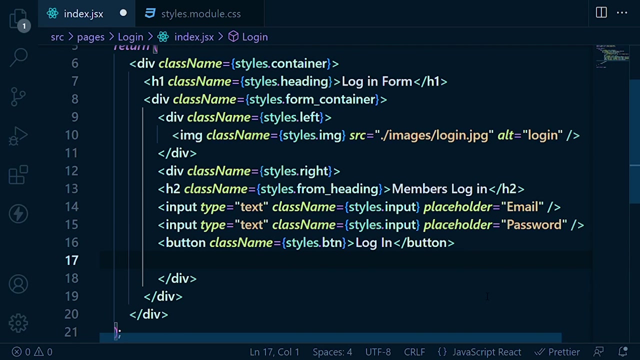 In left div, add image element. provide login image which located in public folders. inside images folder, you can download these pictures from github repo or use different pictures. after adding pictures inside, write div. add heading members login. then add email input and password input. also add login button and or text in p tag after that. 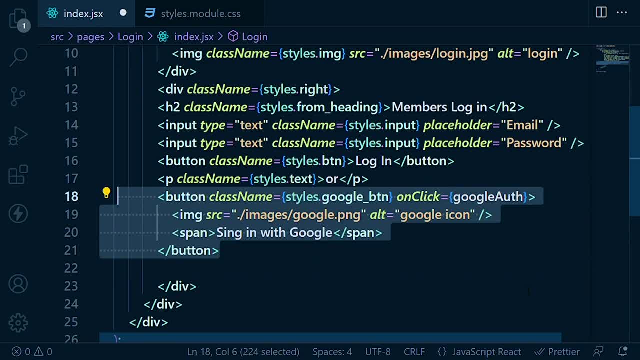 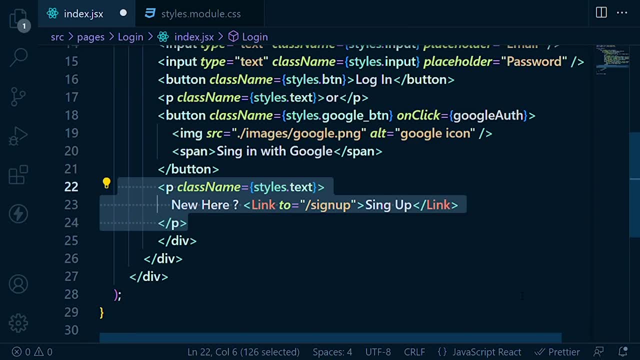 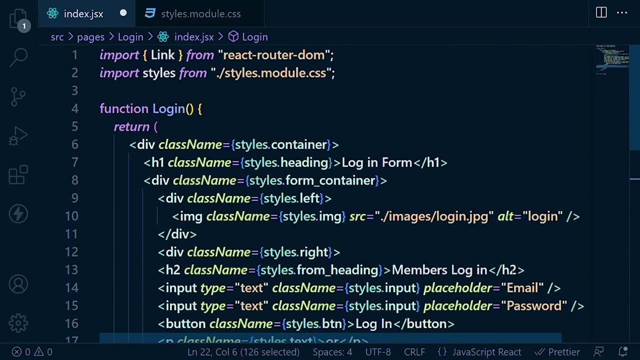 add Google button on click event call Google Earth function, which we haven't created. it. then, at last, add this text in P tag: by clicking signup text we will redirect to signup page without reloading page. that's the speciality of link component. let's create a function named Google Earth inside that function. 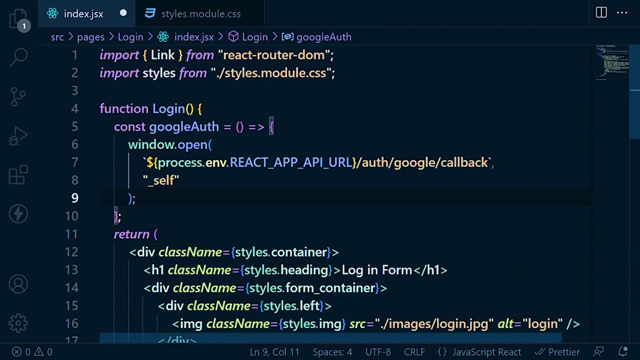 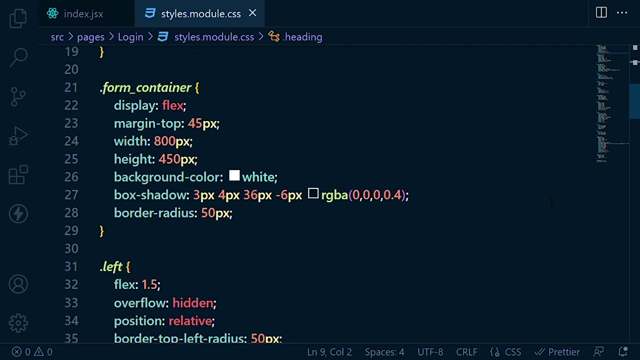 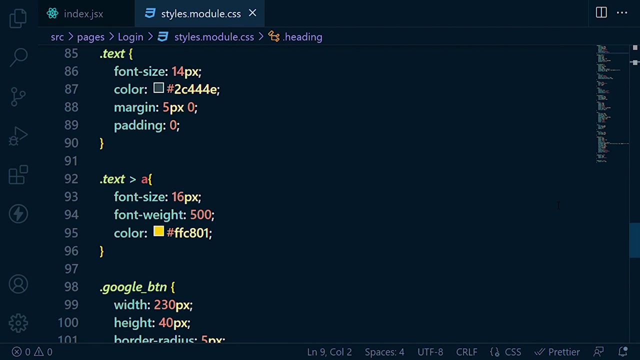 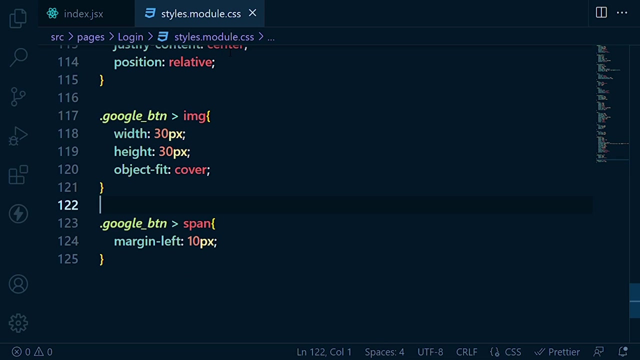 called window dot open method and pass our callback URL. I want to show Google prompt in same page. that is why I am using Google Earth function instead of I am setting self. that's it, guys. save this file now. signup page is almost identical to login page, so without wasting time, let's copy. 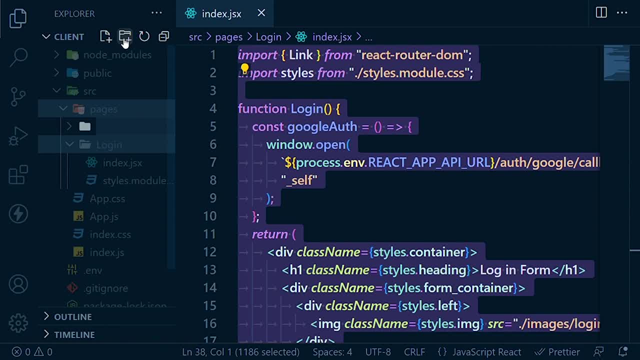 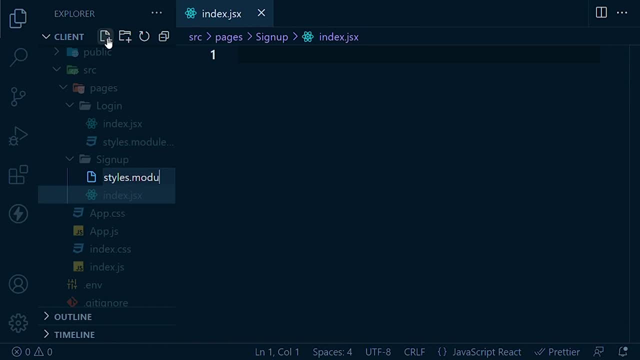 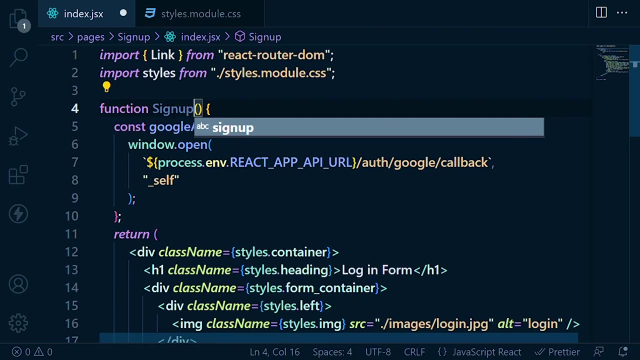 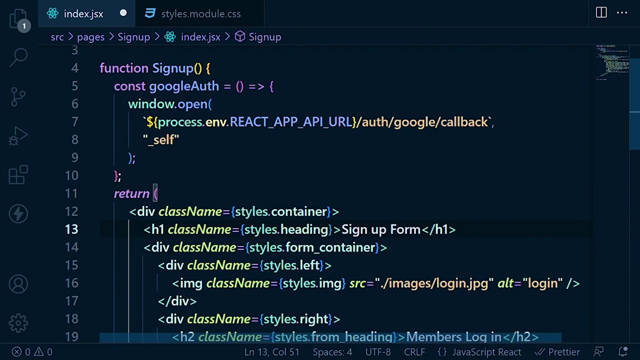 this whole code in this folder. create signup folder inside that folder. create index dot j SX and styles dot module dot CSS files in index dot j s X page. the whole code which we have copied from login page. let's change its name to signup. heading will be sign up, form image will be signup dot jpg and change all text to: 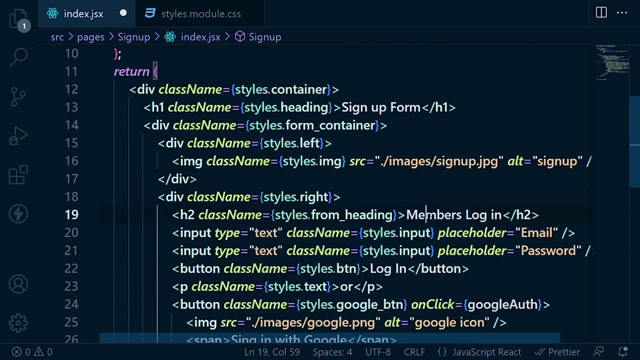 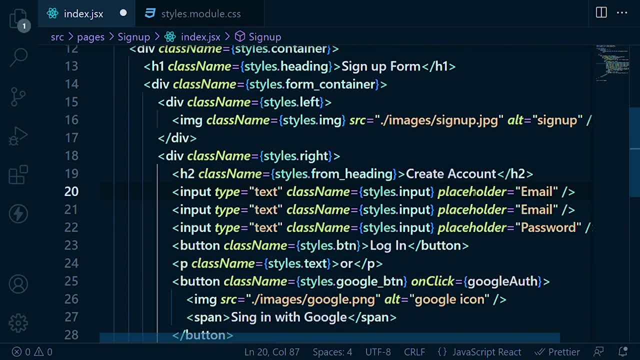 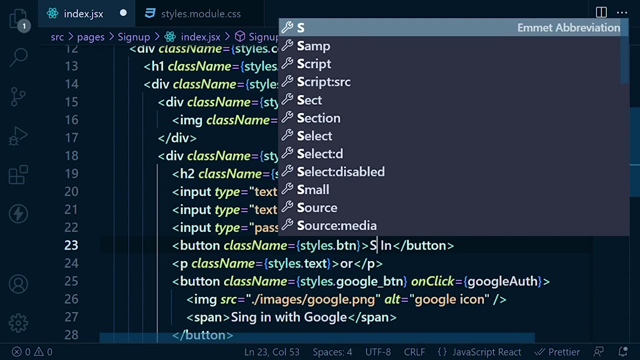 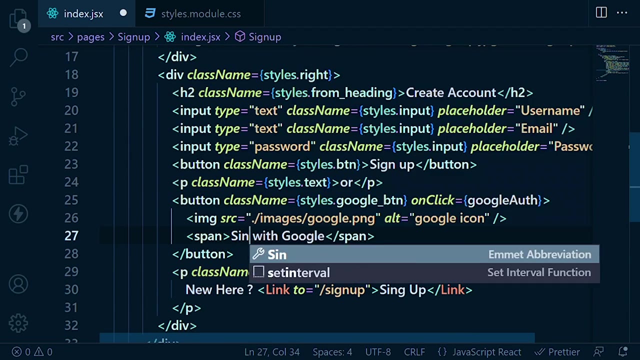 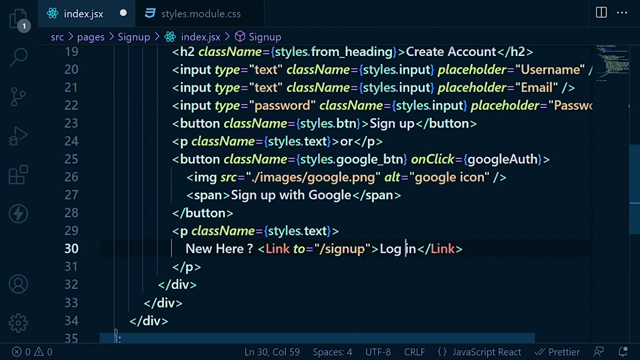 signup form. heading will be create account. We need extra element here for username. Change type to password, for password input, Change login to signup button. Google button will be signup with google. Change text to already have account and let them navigate to login page. 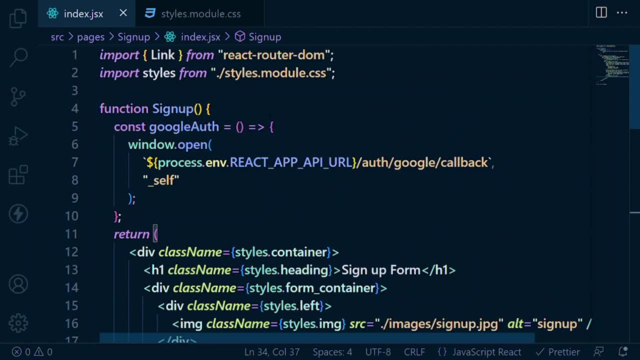 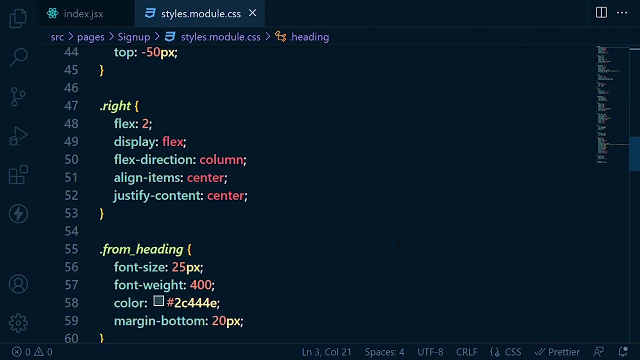 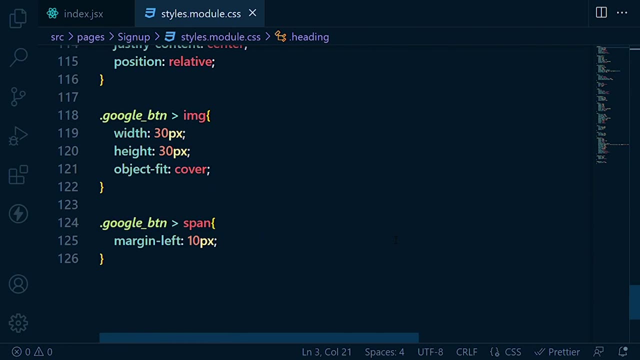 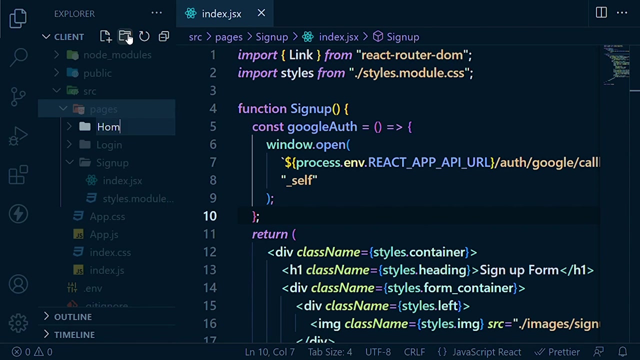 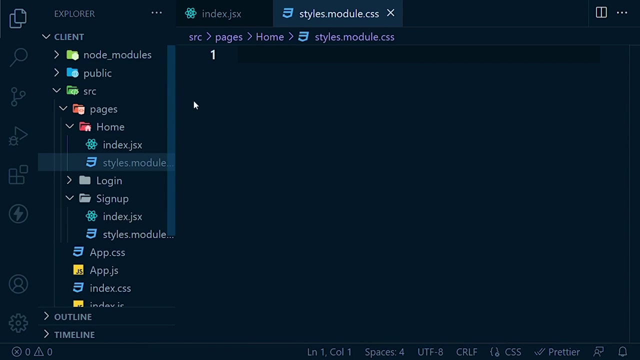 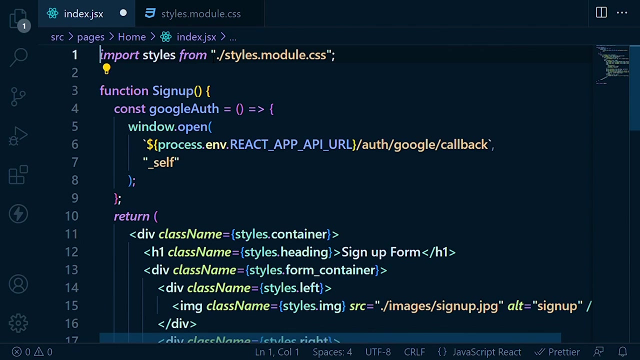 That's it guys. save this file. Let's copy signup component code in pages folder. create home folder. Inside that folder Create indexjsx and stylesmodulecss files. In indexjsx paste the code we have copied from signup page. We don't need link in this component, so remove it. 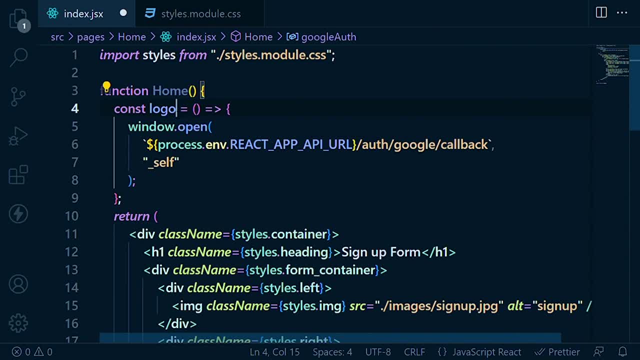 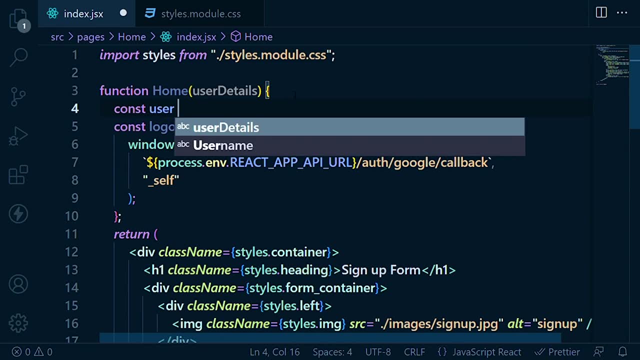 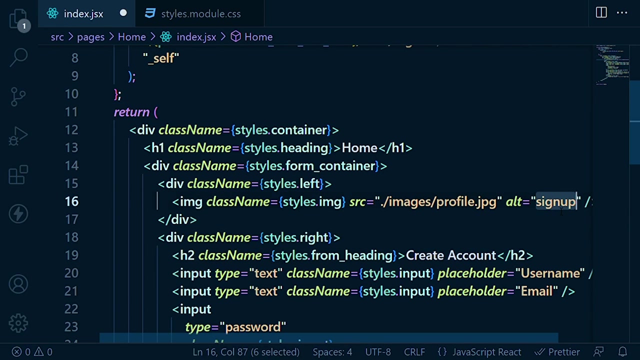 Change function name to home. Change google earth function to logout. We will pass user details from appjs as params user details. Save user details in a variable Here. we gonna call logout api, not callback. Change heading to home. In left div image will be profilejpg and alt will be profile. 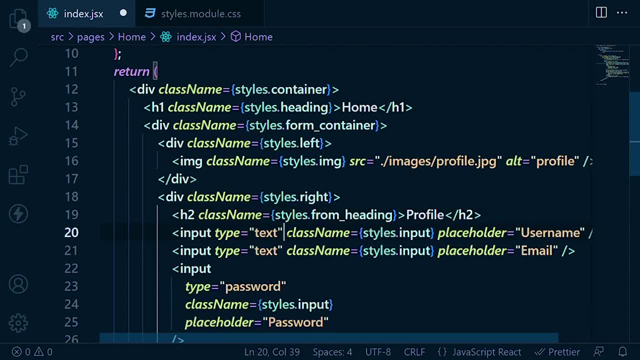 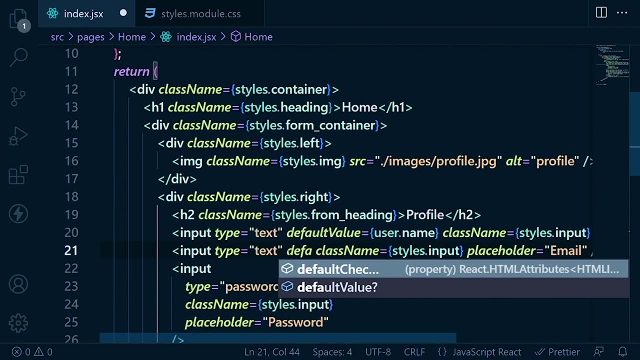 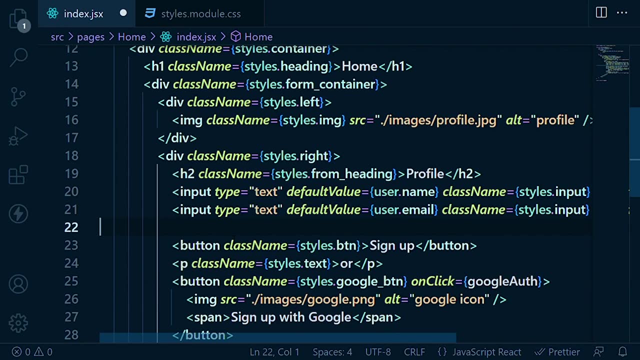 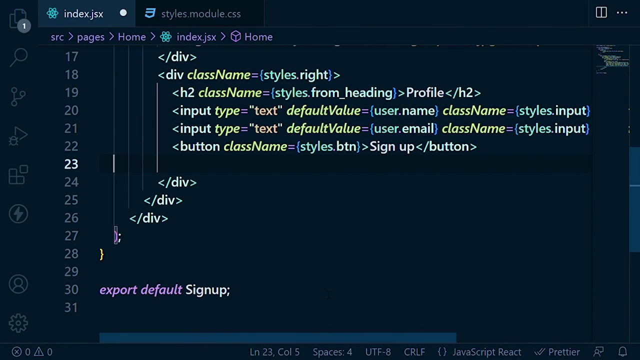 Change form heading to profile. Set default value for username- value we get from user details- and also set default value for email. also Remove password input. we don't required here. Remove this whole code which we don't required. Change signup button to logout button. 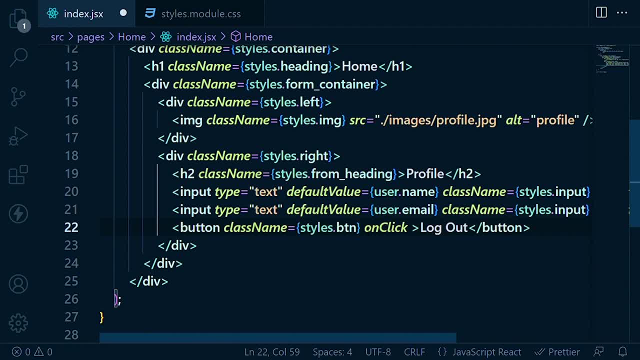 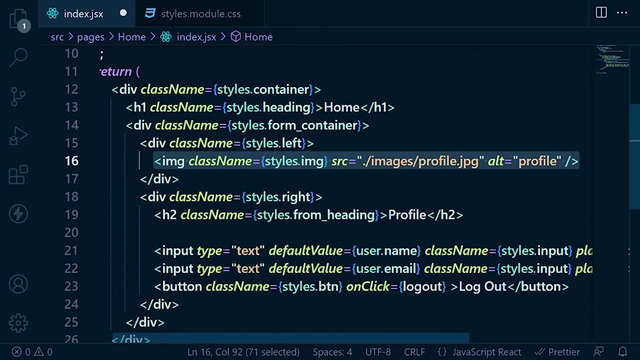 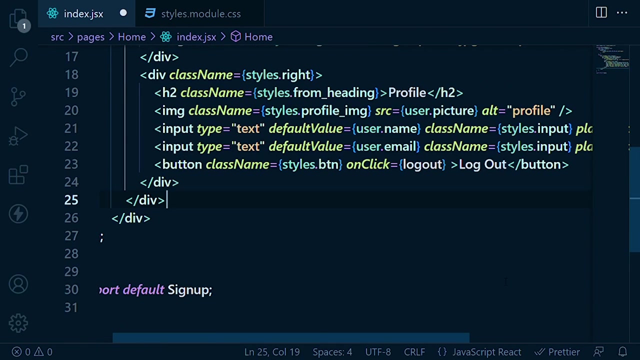 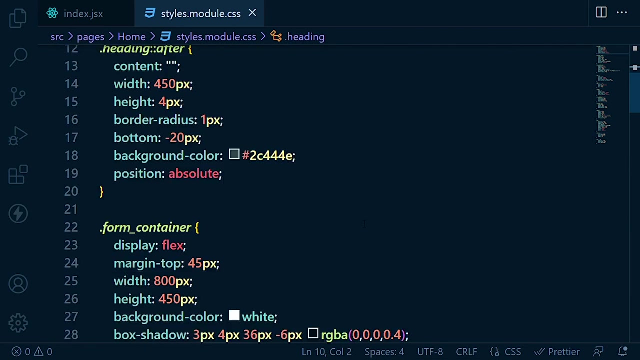 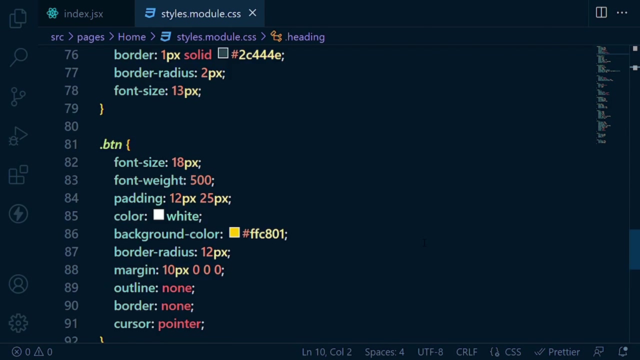 On click event call logout function. Here we also show picture of user, So copy the image element from above. Class name will be profile image And source will be userpicture. Let's export home component. Everything looks fine. Let's save. Now let's open up a appjs file. 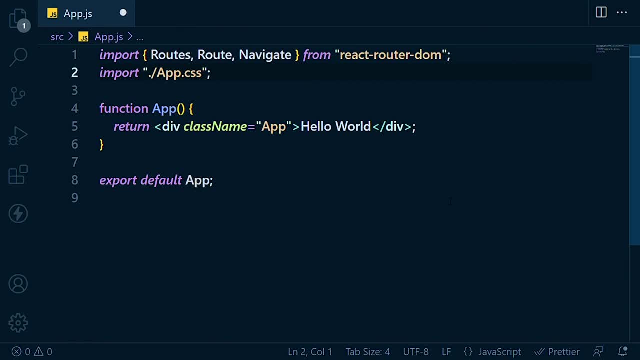 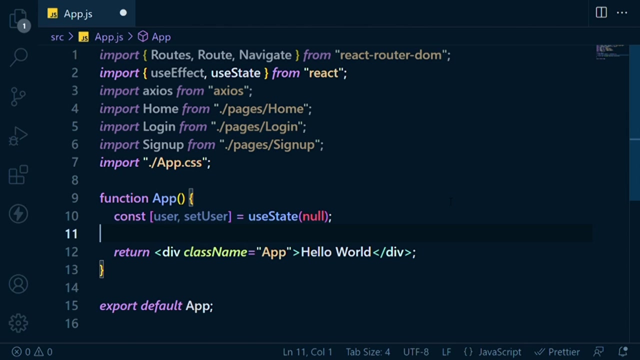 In this file. import router route and navigate from react-router-dom module. Then import useEffect and useState from react module. Import xios from xios. Import home component. Then import login component and signup component. Create state for user and set default value to be null.